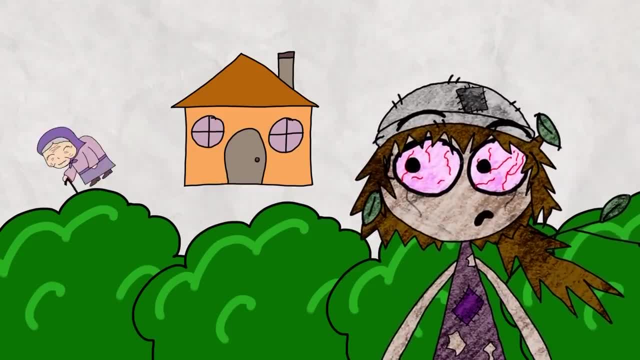 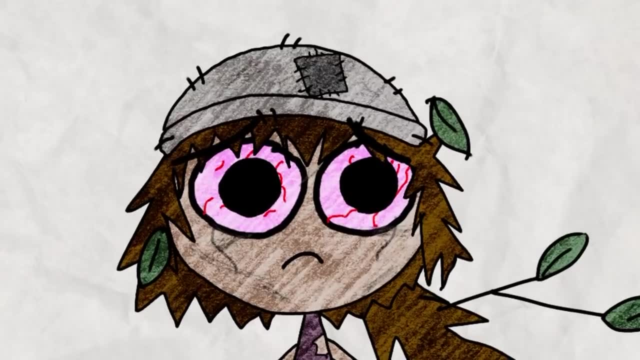 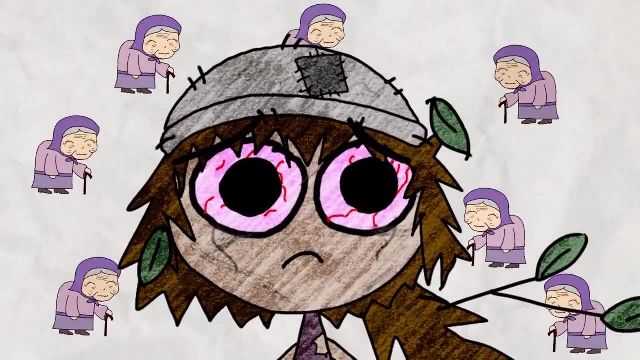 Or what if she needs more cat food and goes twice. Really, you need an infinitely long time to be 100% sure that Mildred frequencies the market once per week. Obviously you don't have an infinite amount of time, So the frequency of Mildred's market trips can never be known to 100% accuracy. 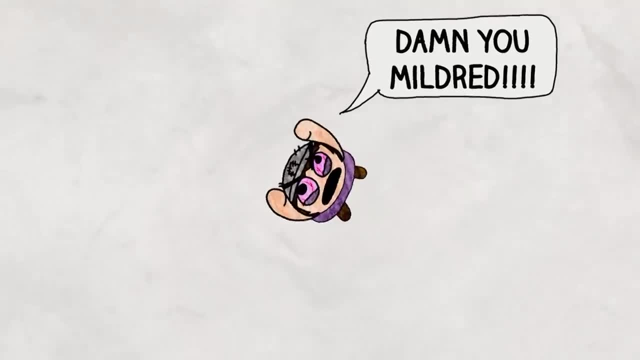 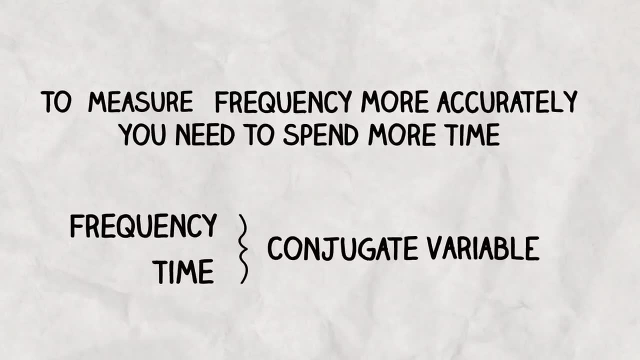 There's this trade-off between knowing the frequency and spending time. This is a version of the Uncertainty Principle, and variables that have this trade-off relationship are called conjugate variables. Another more well-known pair of conjugate variables are position and momentum. 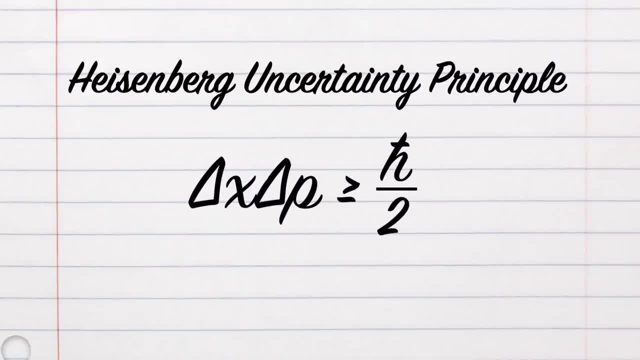 This is one version of the Heisenberg Uncertainty Principle, and it states that the uncertainty in position and the uncertainty in momentum are always greater than or equal to this constant. here, Basically, we can never measure both the position and the momentum of an object to 100% accuracy. 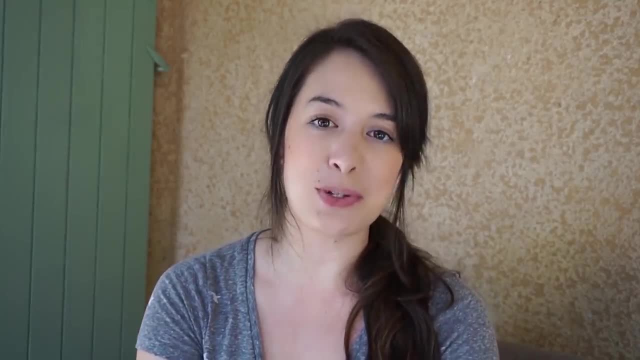 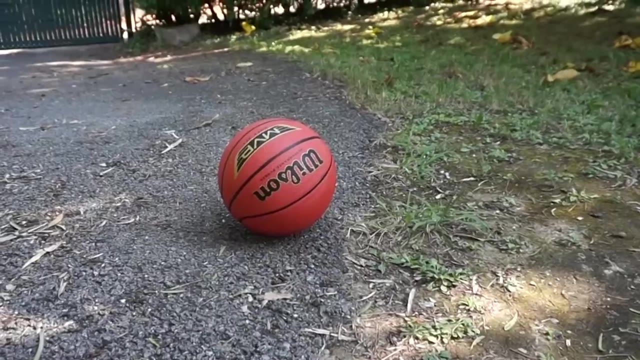 We'll come back to the equation in a bit, but first let's talk about the intuition. The way my quantum physics professor introduced the Uncertainty Principle was: imagine you're trying to find the location of a basketball. but the only way you can do that 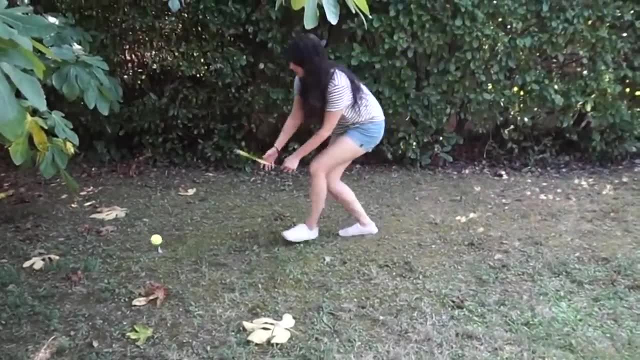 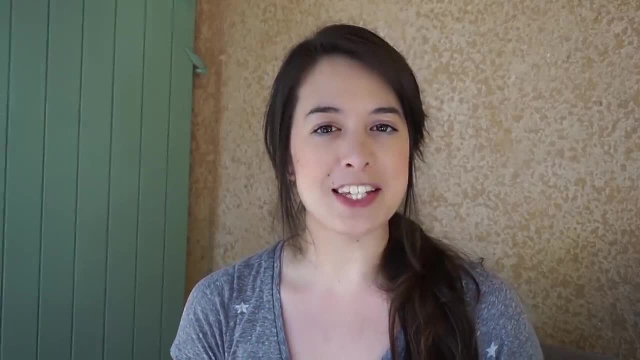 is by throwing tennis balls at it and measuring where they bounce back. If you manage to hit the basketball, sure you know where it was, but now it's moved. Keep the imagery in mind for this next bit. Heisenberg was a German physicist who loved. 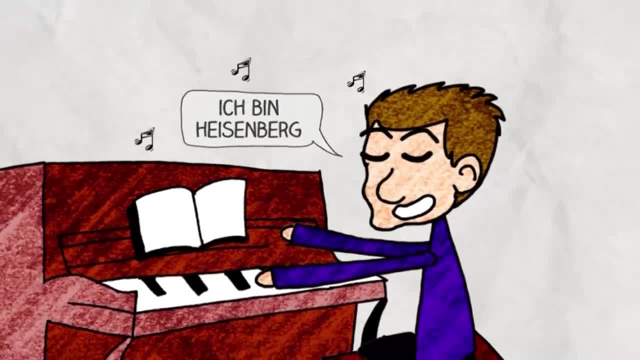 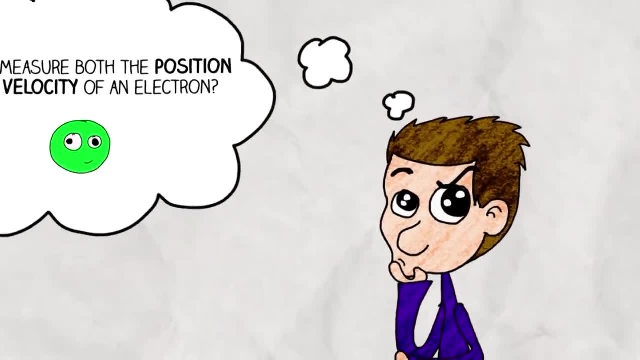 classical music and was a pretty accomplished piano player. Oh yeah, and he won the Nobel Prize for the creation of quantum physics. One day he was performing a thought experiment. He wanted to see if he could measure both the position and velocity of an electron. 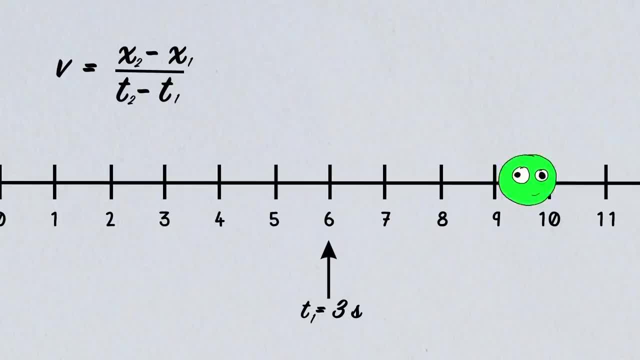 To measure the velocity of something, you just need to measure its position twice and divide by the time it took between each measurement. So it seems silly that you could measure something once but not twice, right? But the most direct way of measuring where something is is to shine. 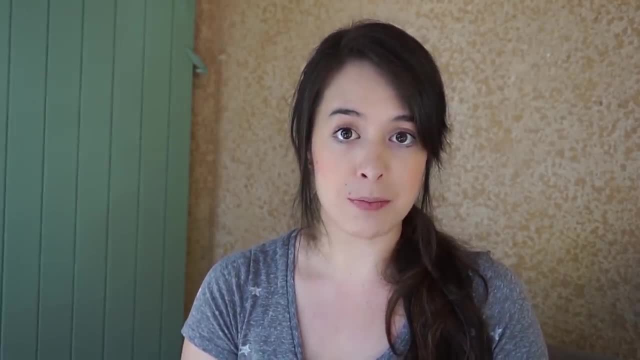 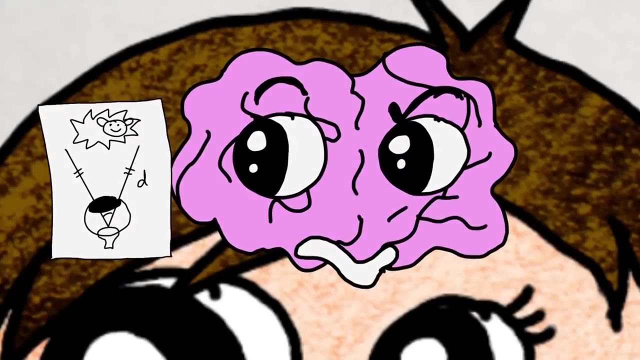 light on it and from the reflected light calculate its position. We do this every day when we look at things. Photons hit the object and reflect them back into our eyes. Then our brain figures out where it is from the image produced on the retina. So Heisenberg imagined. 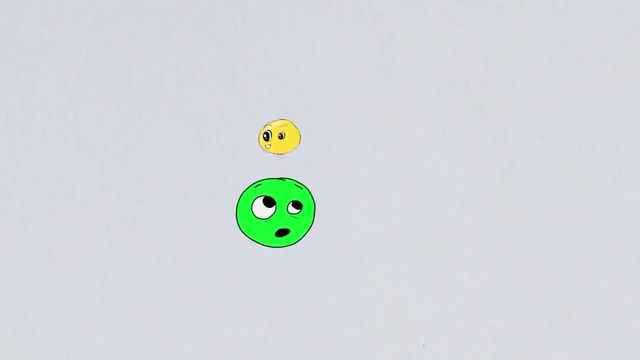 looking at an electron under a microscope, firing a photon at it and figuring out the position of the electron. But in order not to move the electron he would need to hit it with a photon of really low energy. Now quantum particles have a property called wave-particle duality. 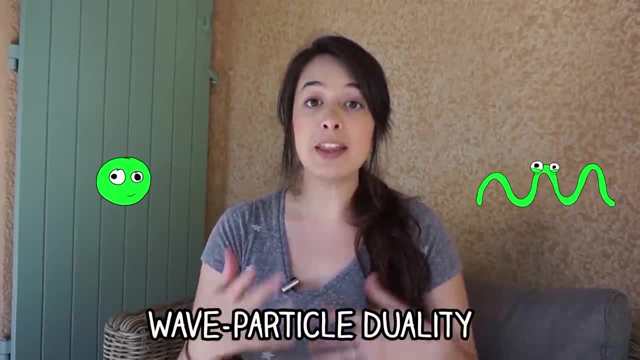 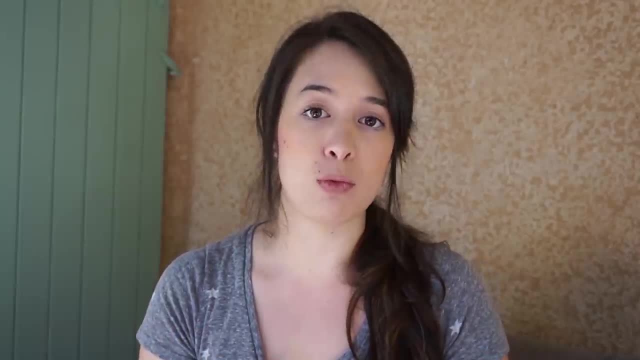 Where they behave as both particles and as waves. So while they can be thought of as particles, they also have a wavelength and frequency. Radio waves have the longest wavelength- 30 centimeters or more- and they're great for capturing images of stars and planets. 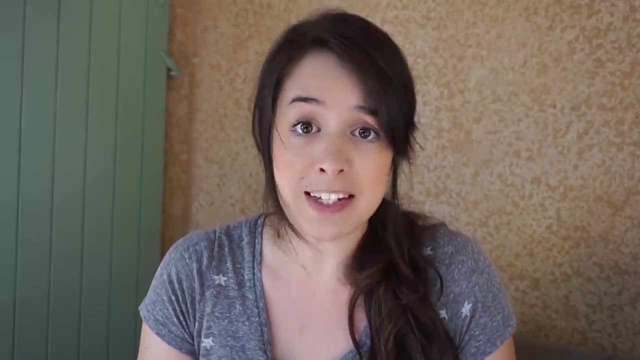 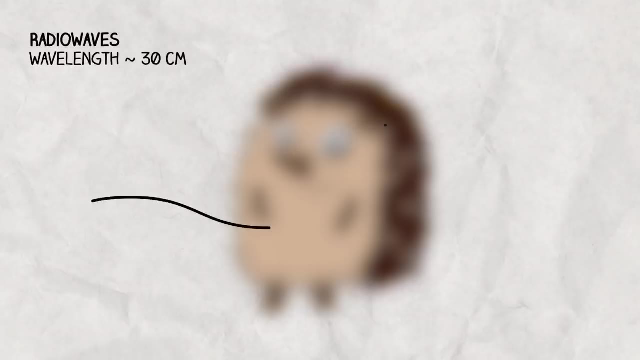 But they'd be hopeless at producing a good image of, say, your face. You would just get a blur. See, you can't get better focusing power than the wavelengths that are forming on the image. The 30 centimeter radio waves can only make images of details at least 30 centimeters big. 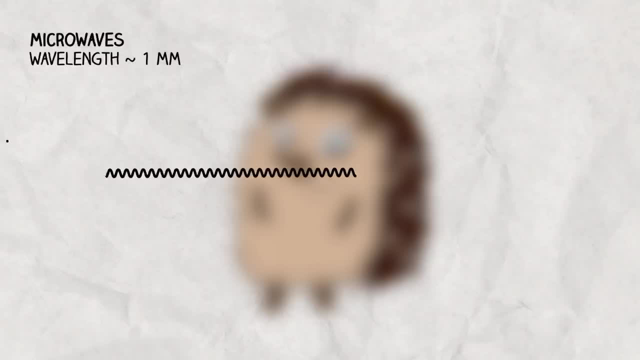 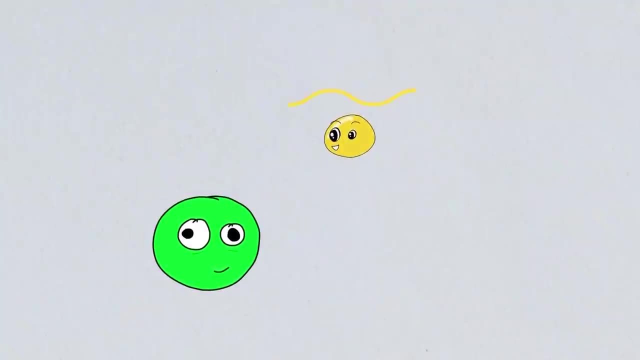 If you made the wavelength smaller to about a millimeter, then you'd get a much better image. So if Heisenberg wanted to get a clear image of an electron, say, to within a micron, he'd need to decrease the wavelength of the photon to within one thousandth of a millimeter. 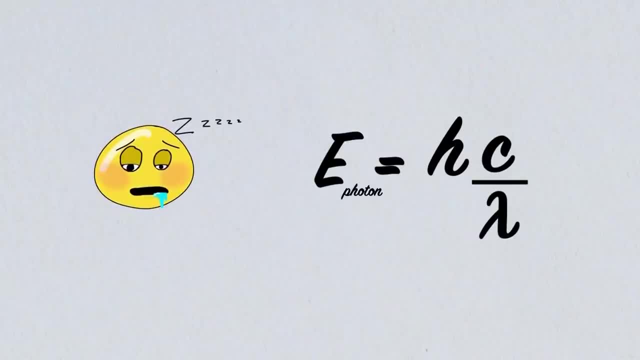 But the energy of a photon is given by this equation, where E is the energy and lambda is the wavelength. So you can see that as the wavelength gets smaller, the energy gets bigger If we decrease the wavelength, allowing us to get an accurate description of its position. 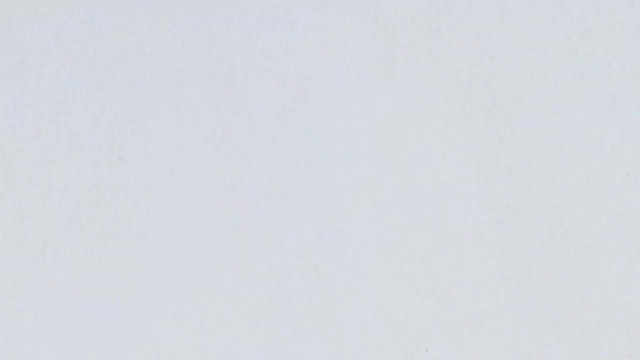 the photon has to be of such high energy that it hits the electron too hard and moves it. If we hit the electron with a photon of low energy and then hit it again, we can get an idea of the velocity, but the images will be too fuzzy to measure its position. 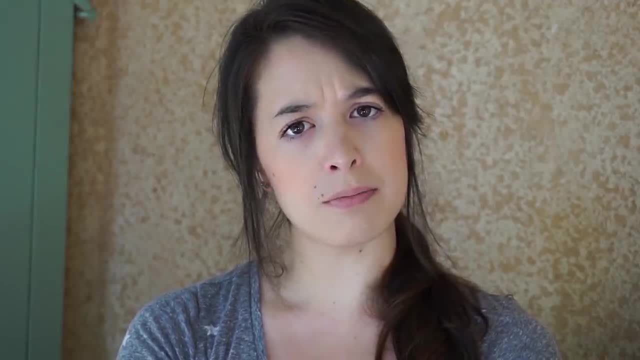 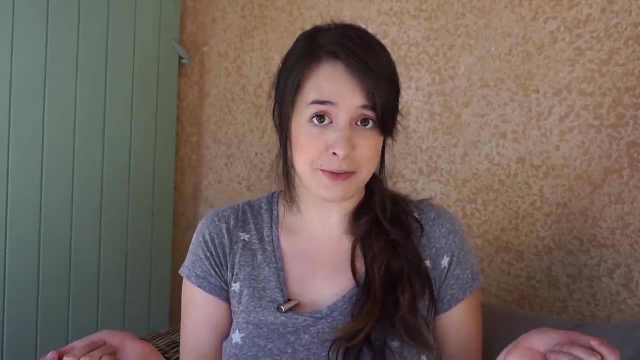 with decent accuracy. This is a conundrum. Position and momentum are conjugate variables. You can't gain information about one without losing information about the other. Now let's go back to our equation. Hopefully now it makes more sense. These triangles mean uncertainty. 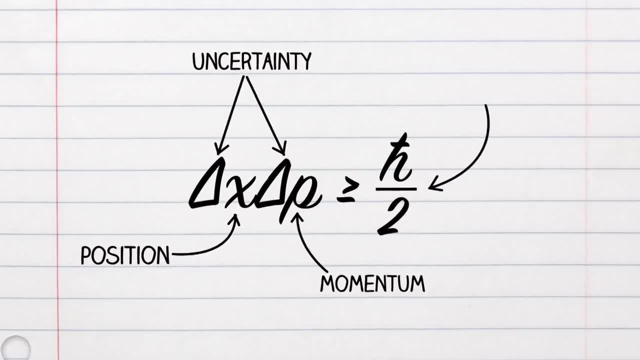 and this x means position and this p means momentum. This h-bar on 2 is a teeny tiny little constant. Don't worry about the exact value right now. The important thing is that it's greater than zero. So the equation tells us that the uncertainty in position and the uncertainty 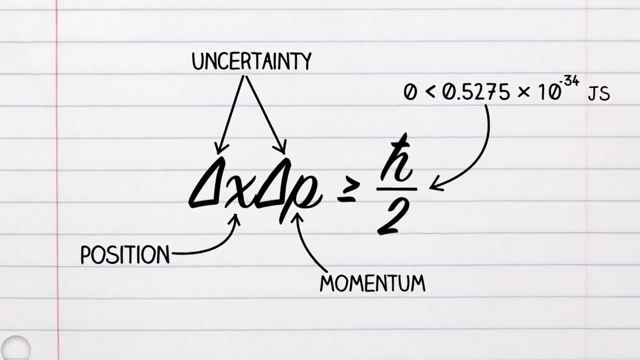 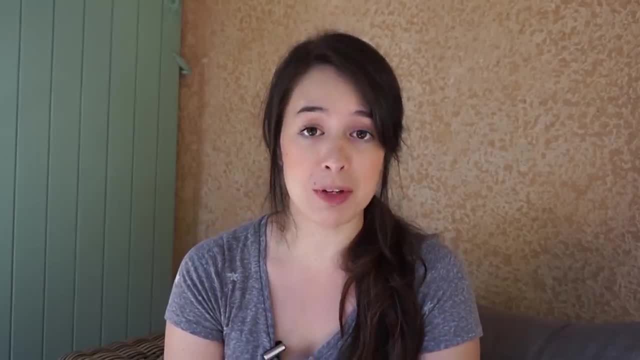 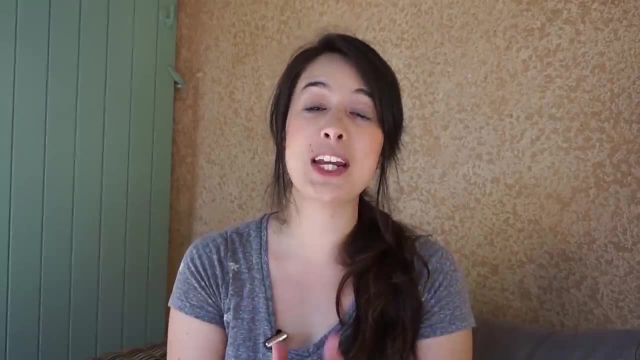 in momentum is always greater than zero. Basically, we have to have some uncertainty somewhere. As we saw from Heisenberg's experiment, this had nothing to do with the equipment he was using. Unless we find a way to make wavelengths shorter without increasing energy, we're screwed. Now for those of you who 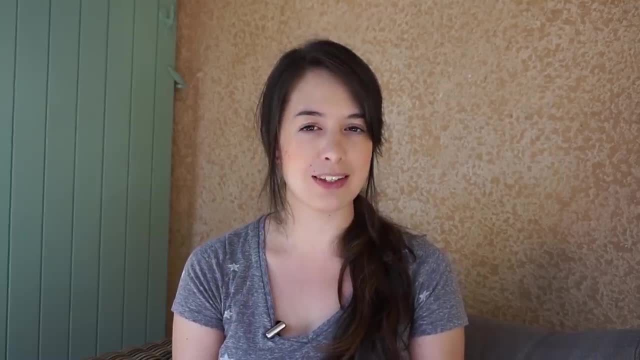 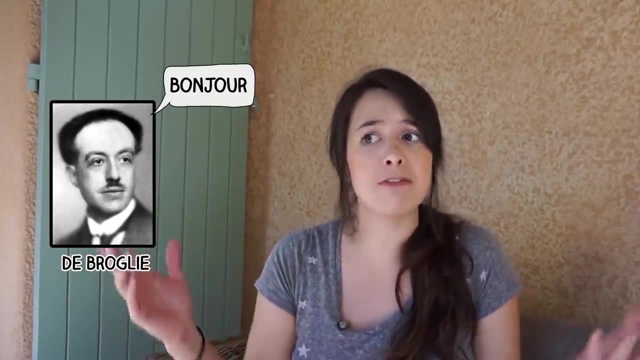 need a mathematical description to go with the intuition. don't worry, it's coming. When Einstein concluded that light behaved as particles, this French guy named de Broglie made this outrageous. totally not founded on anything claim that all particles must behave like waves. 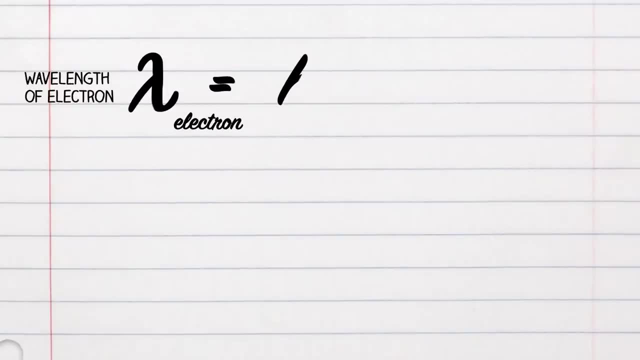 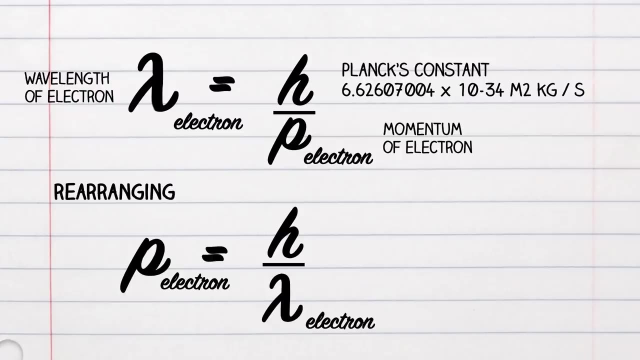 too, And he was right. The wavelength of an electron is just Planck's constant, divided by its momentum. Therefore the momentum of a wave can be represented by a wavelength. So say, we know the exact momentum of an electron. We can represent it as a beautiful 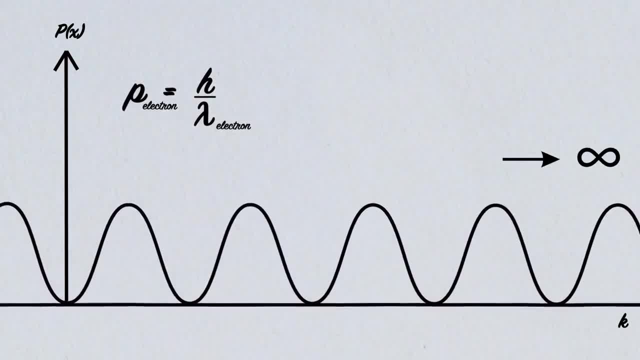 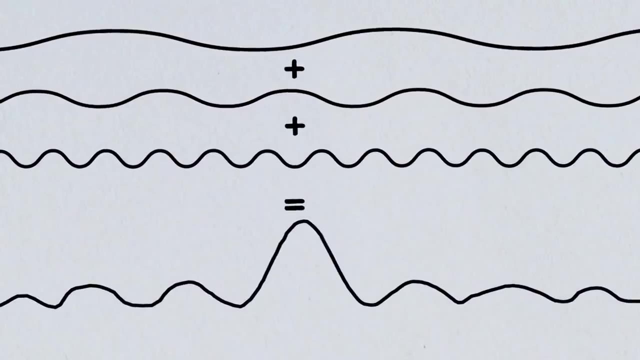 infinitely long sine wave. But the position of the electron is also described by this wave. The area under the curve represents the probability of it being there and we can see that we have basically no idea where it is. But waves have this cool property that when you add them together they interfere and create a new wave. So say we present: 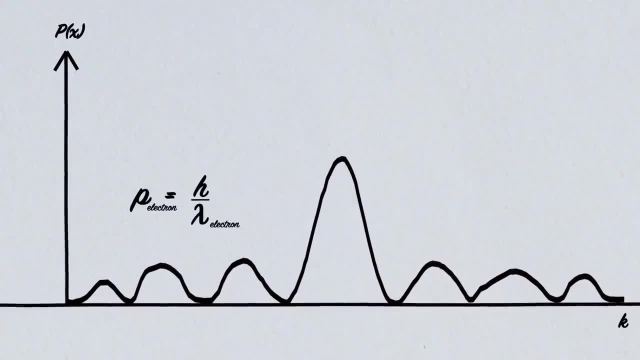 a stillכrong�ацион Bitte dialect of a special book with different wavelengths And immediately, what we're describing is that wave that describes the electron's position and momentum. Now the electron is much more localised and we have a way better idea of where it is, But this wave is made up of a sum of a. 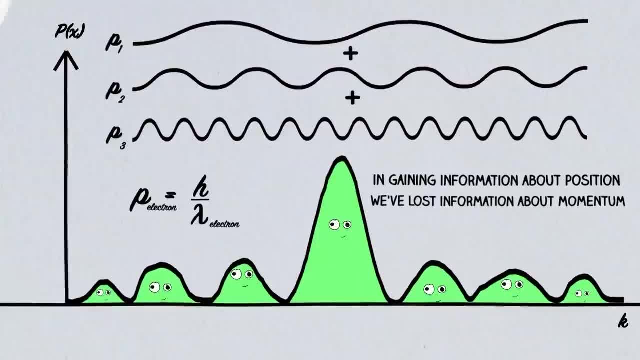 lot of different wavelengths, And remember that wavelength and moment gal are practically interchangeable. So then we no longer have just one momentum value, we have loads. So in gaining information about the position of the electron we've lost information about its momentum. Position and momentum are just two of loads, of different wra Gordon contingencies. 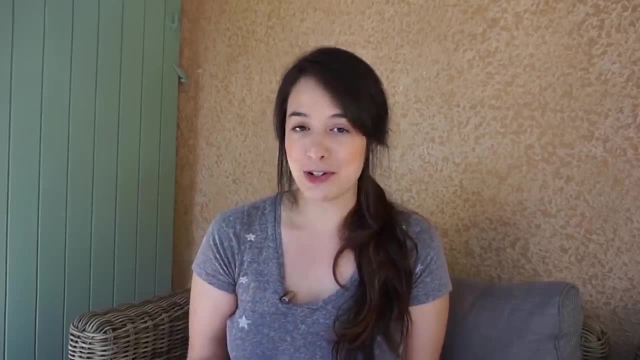 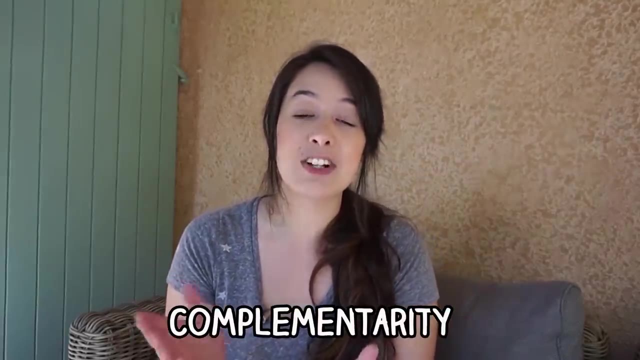 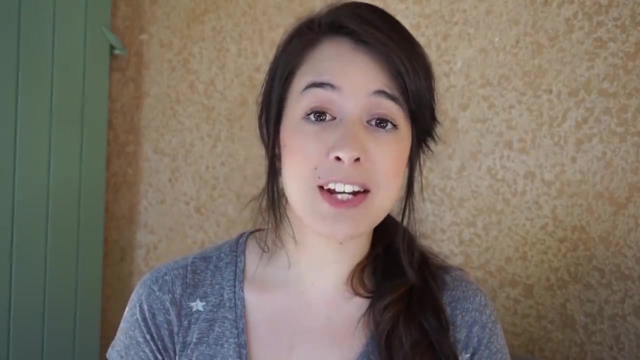 conjugate variables. Heisenberg's mentor, Niels Bohr, gave this relationship between conjugate variables a proper name: complementarity. The deeper meaning is that there are some pairs of complementary properties that just can't be measured or observed simultaneously. Trade-offs are built into the laws of nature, the particles that make up our universe. 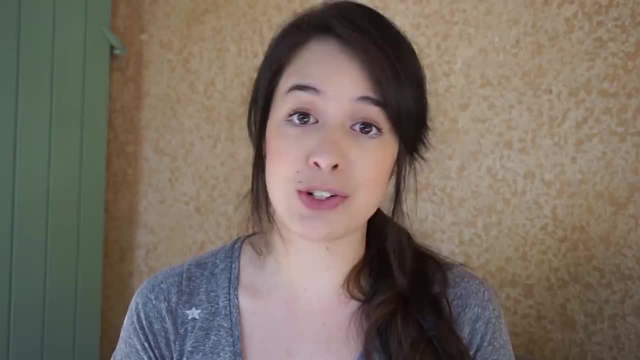 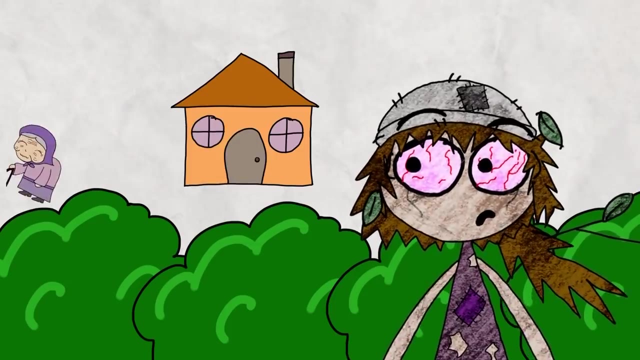 and our lives. So next time you think you can have your cake and eat it too, you probably can't. I'm often asked how I make the animations for my videos, and the answer is that I use Adobe After Effects. For anyone wanting to learn to animate, Skillsharecom is a learning website.